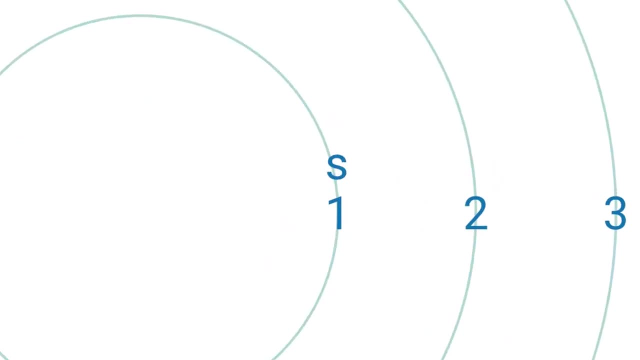 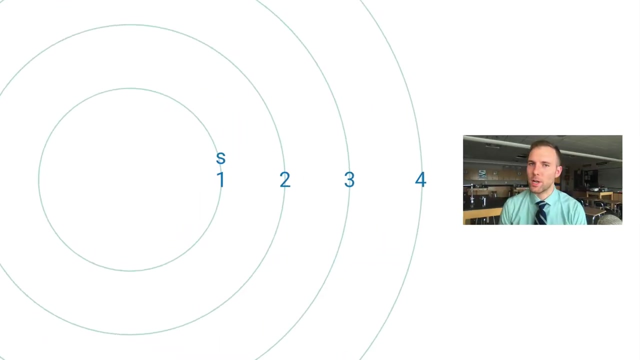 nucleus has only one, what we call S subshell. A subshell is something that's contained within a shell, and each shell has at least one. Now, the first shell only has one. The second shell has an S subshell, but it also has a P subshell, which is a little bit bigger. 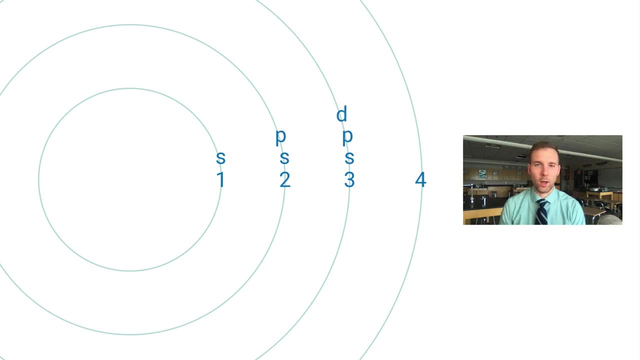 The third shell has an S, a, P and a D subshell. A D subshell is even bigger than a P. And then the fourth shell has four subshells in it. It has an S, a, P, a D and an F subshell. 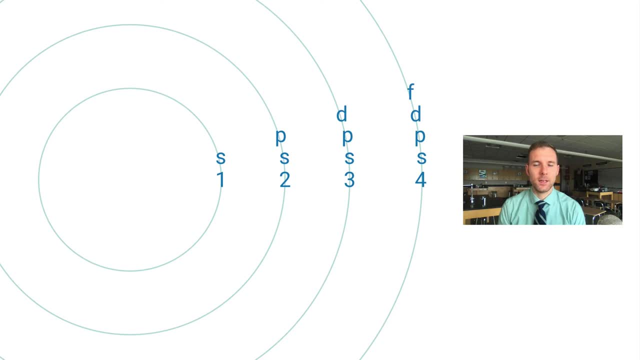 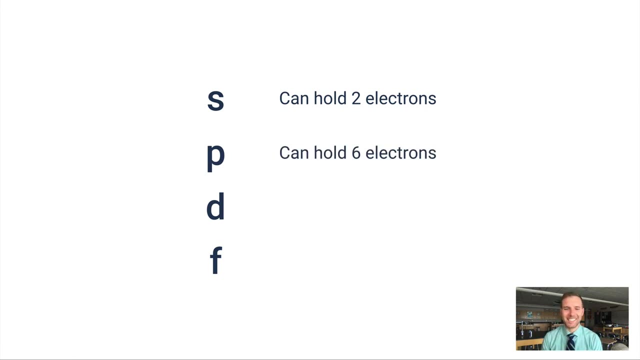 And of these four subshells, F is the biggest. So let's look at this a slightly different way. An S subshell can hold only two electrons. a P subshell can hold six. a D subshell can hold ten electrons. 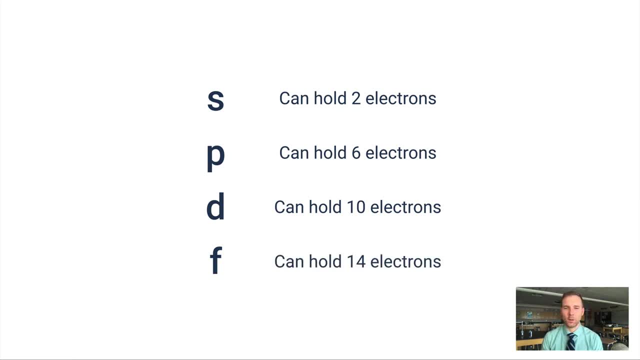 and an F subshell can hold fourteen. Now, if you look closely, there's a a bit of a pattern here. As we move from S to P to D to F, we're able to hold four more electrons than the previous subshell, And there's a reason for that. Each subshell contains a certain number of orbitals. 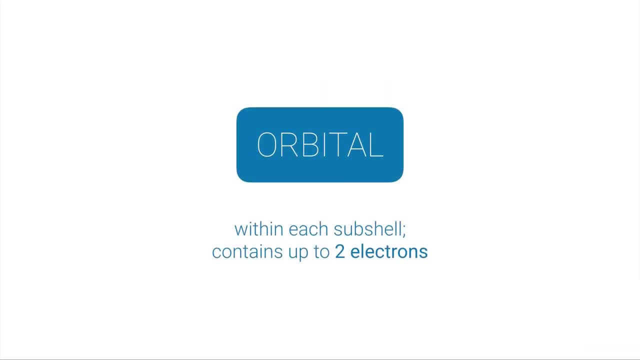 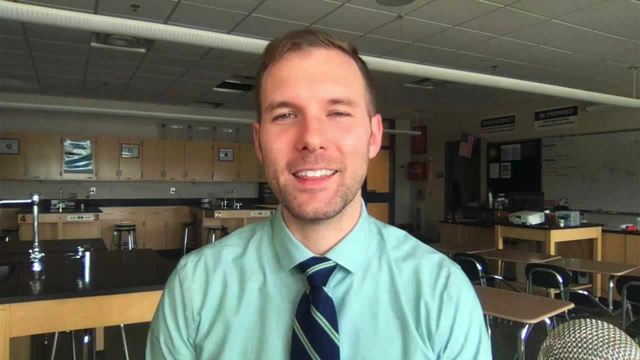 An orbital is something within a subshell that contains up to two electrons. Okay, so let's pause for a second and take inventory of all the information that we just heard. We heard that the D subshell contains a certain amount of electrons, So the number of electrons is one-third greater than the number of electrons. 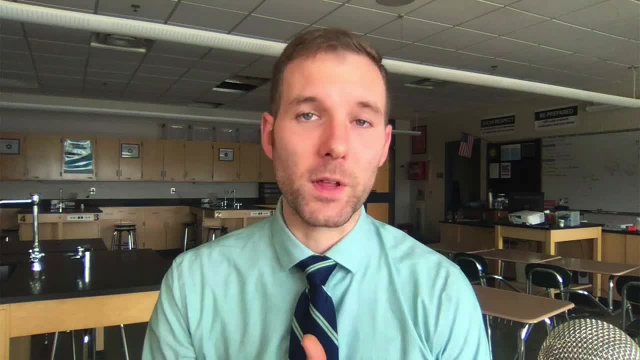 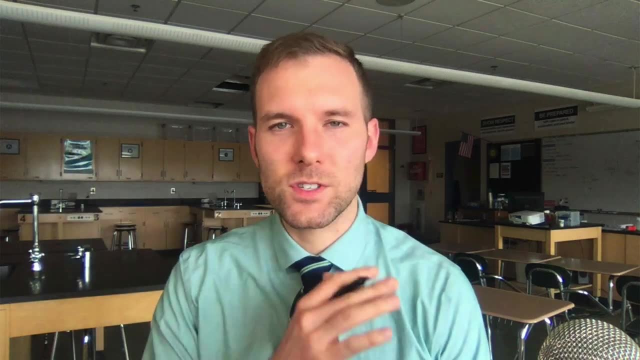 Okay. so let's pause for a second and take inventory of all the information that we just heard: that there are seven shells around a nucleus. This is where the electrons live, But within each of the seven shells there's a different number of sub-shells And within each of the 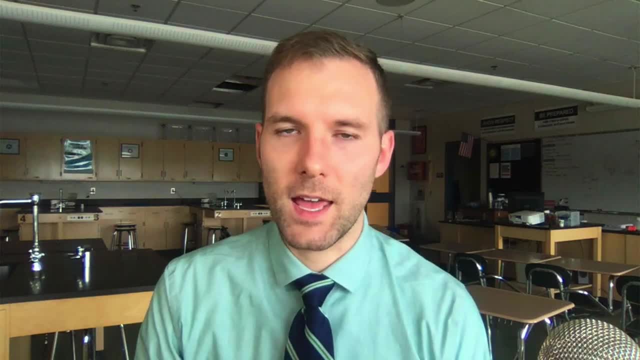 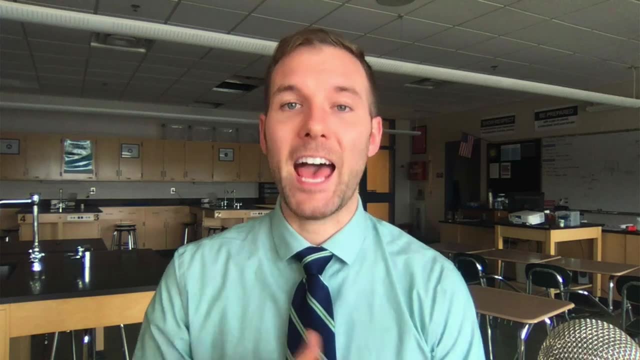 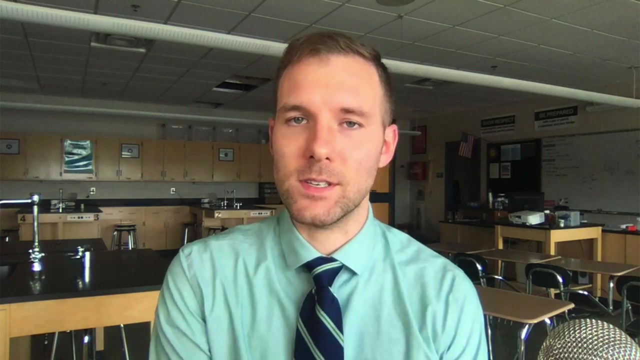 sub-shells, there's a different number of orbitals, And orbitals are really where the electrons can be. Think of it this way: A shell could be like a town, A sub-shell could be like a road in that town And an orbital might be one of the houses on that road in. 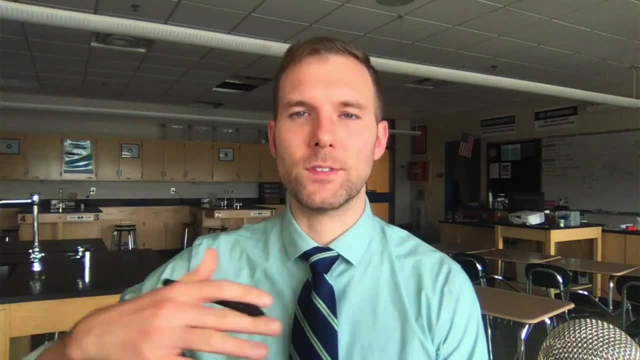 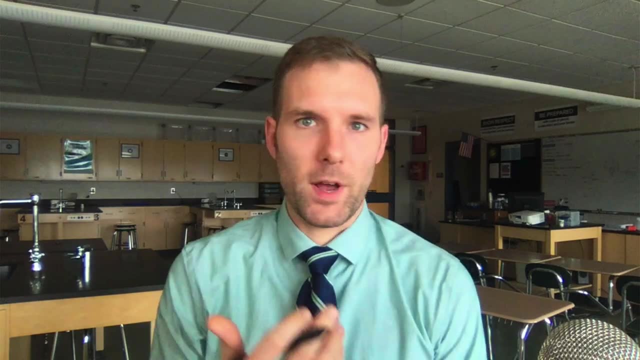 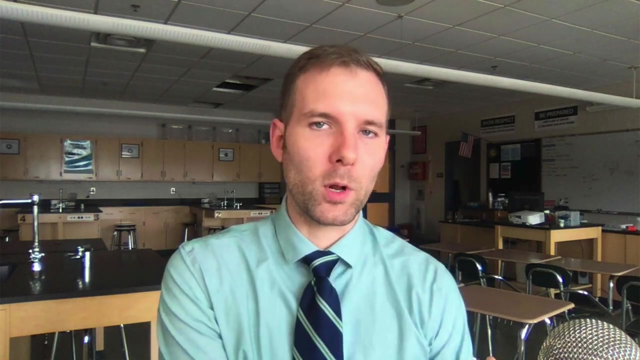 the town. You can see, as I kind of zoom in from shell to sub-shell, to orbital, I'm talking about a more specific location. An address has a number on a street in a city, And so you can think of an orbital as the number, the sub-shell as the street and then the 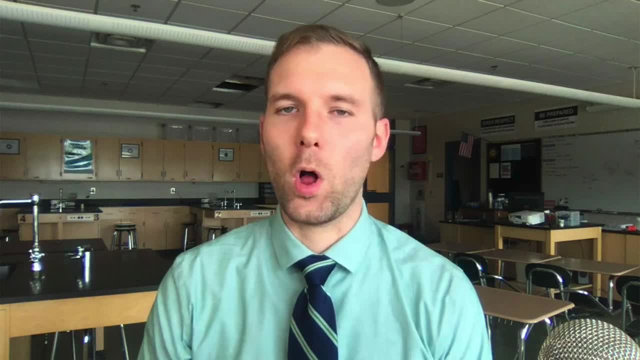 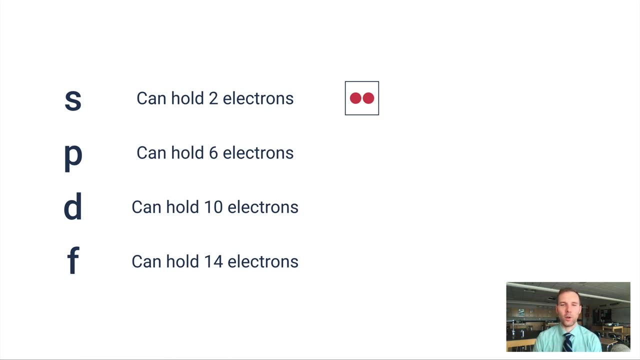 shell Itself, one through seven, as the city where all of this is located. Hopefully that helps. Now let's continue. The S sub-shell has only one orbital, And if only one orbital can fit two electrons, then the S sub-shell can only fit two electrons in it. The P sub-shell has 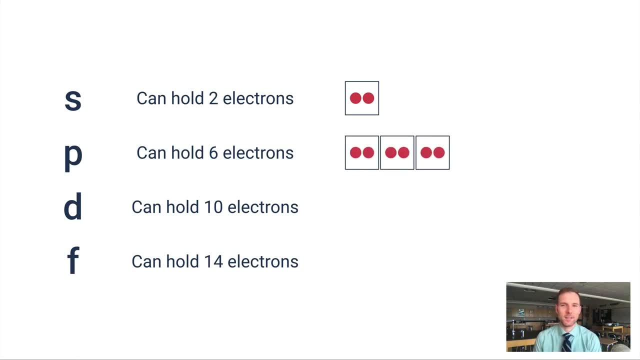 three orbitals, and that's what allows it to fit six electrons. Two orbitals or two electrons per orbital. three orbitals two times three is six. The D sub-shell has five orbitals, That's ten electrons, And the F sub-shell has seven orbitals, which would equate to fourteen electrons room. 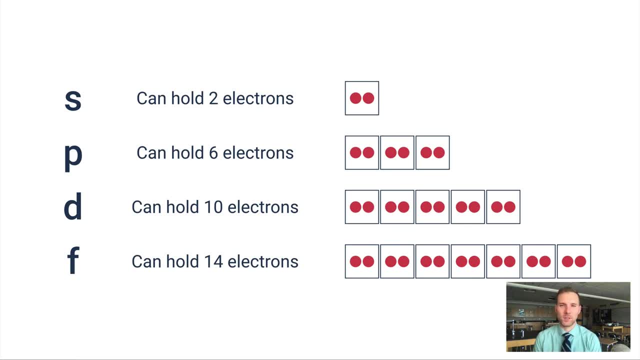 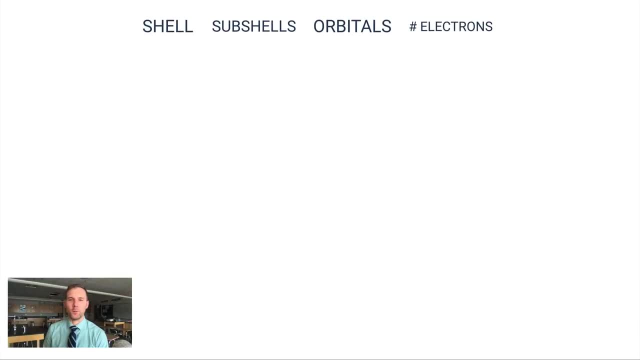 for fourteen electrons. These are all the maximum amounts of electrons that can fit in each of these sub-shells. Okay so let me show you this a slightly different way. A table comparing shells, sub-shells, orbitals and number of electrons. And in our first shell we only have an S sub-shell. 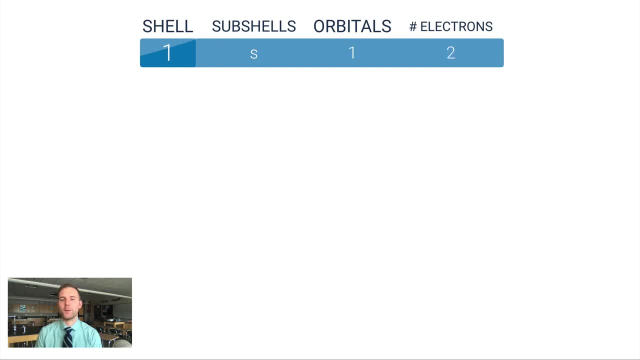 which means we only have one orbital on the first shell, And that's why in the first shell we can only fit two electrons. the maximum amount of electrons in the first shell is two. i could have zero or one, but i can't have. or i could have two, but i can't have more than two in this second. 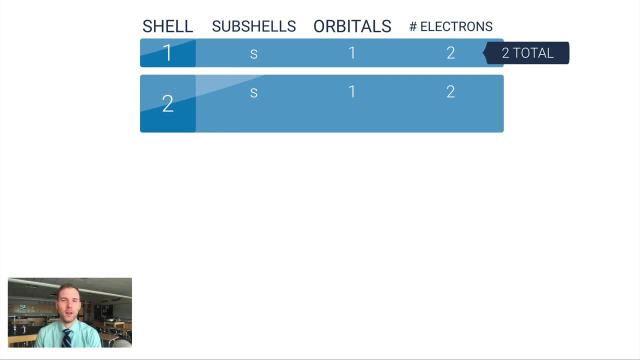 shell. i have an s subshell, just like i do in the first shell, but there's also a p subshell which has three orbitals in it, and that means it can hold six electrons. now if you add two and six together for the second shell, you end up with eight total electrons that can fit in the second. 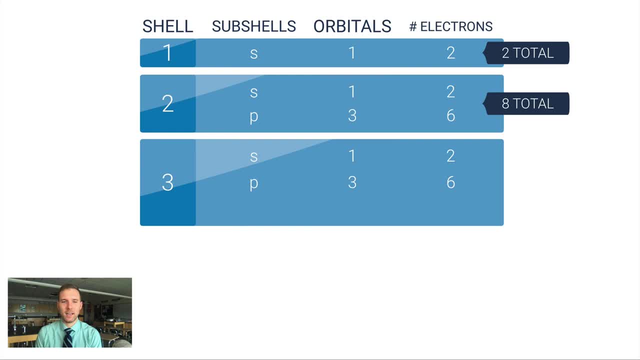 shell. let's move on to the third shell. i have an s and a p, just like the second, but this also has a d subshell which has five orbitals in it and therefore can hold 10 extra electrons. now, 2 plus 6 plus 10 makes 18.. i think you can see where i'm going with this. let's do the fourth shell just. 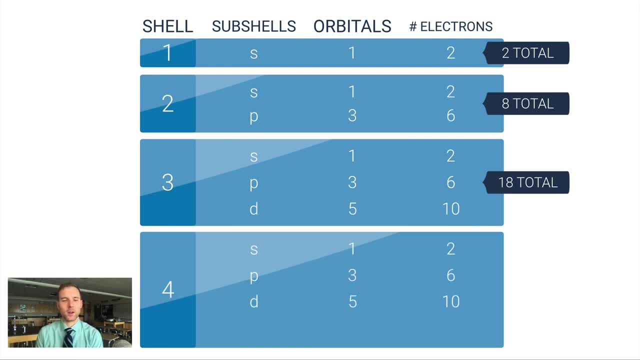 for good measure. that has an s, a p and a d. it also has an f, which is seven orbitals and therefore can hold 14 electrons. if you add up 2, 6, 10 and 14, you get 32, and these numbers here should probably be pretty familiar to you, if you're. 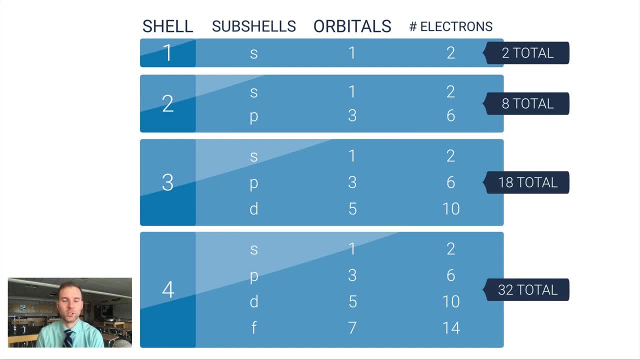 thinking of, kind of the first explanation of electron configuration: 2n squared, where n is the shell number. that's where that trick comes from. it's this. we really have this going on in all of these shells. so let me show you an orbital filling diagram. this is a 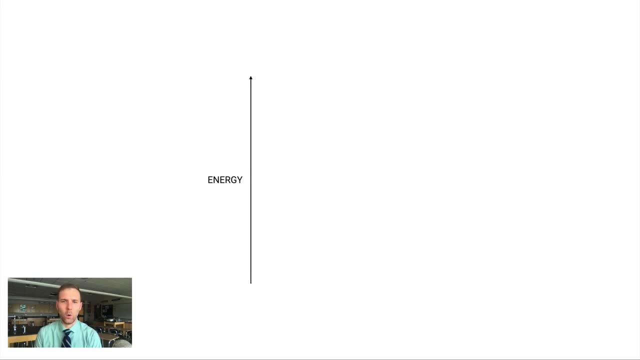 you can think of it like it's a chart that really only has a y-axis and that's that the lower you are in the chart, the less energy you you needed or you need to have in order to be there, the higher up you are. if you're an electron, that means you have to have a lot of energy to be there. 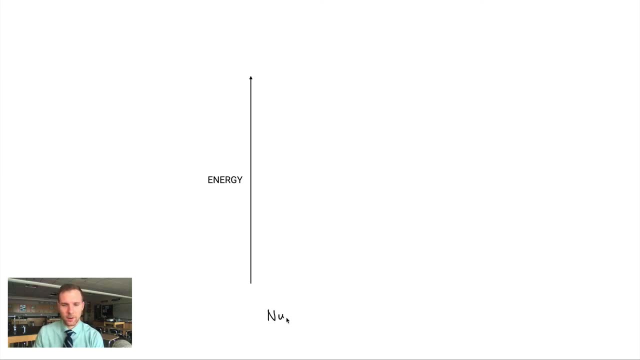 now think of it this way: the nucleus is down here. so this is where the nucleus is. and then the first shell, remember, just has one subshell and only one orbital in the that subshell. that's the 1s subshell. that's got the lowest energy. if you're an electron and you're 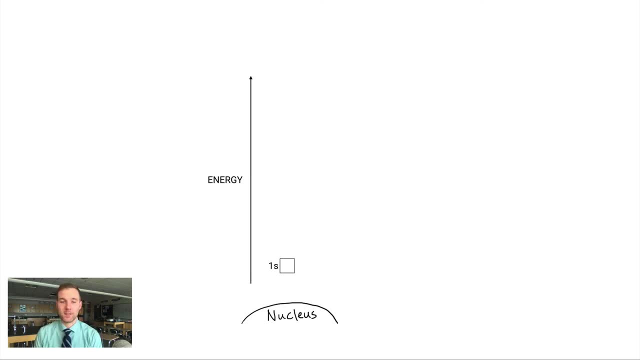 very close to the nucleus you don't have a lot of energy. so the second subshell, the 2s subshell, is a little bit further out and so it requires a little bit more energy to be there. the 2p subshell with its three orbitals it's pretty close energy wise but it actually requires. 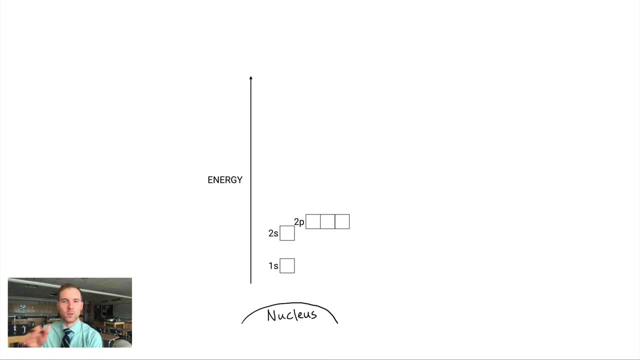 more energy to be in the 2p subshell, even though you're still talking about the same second shell, that second ring outside the nucleus. there are delineations now, all the orbitals in the 2p subshell, all of these here. these are all at the same energy level, but 2p requires more energy than 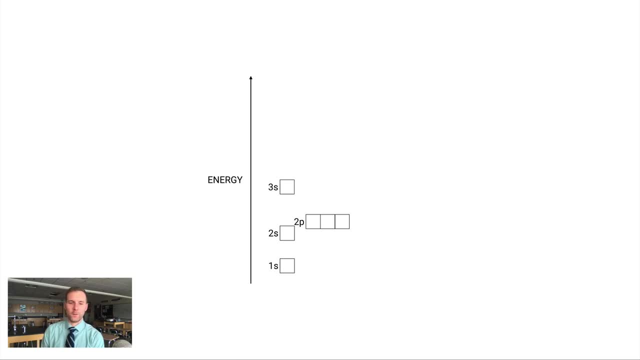 2s does. let's keep going. now we've filled our our second shell, we've run to the third shell, 3s and 3p, and it's business as usual so far. but something strange happens right about here. you'd think that the 3d subshell would be the 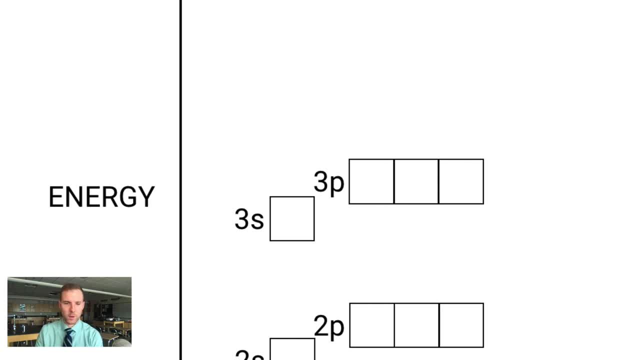 next subshell that would pop up because, if we're following our pattern, we have 1, 2, 1s, 2s, 2p, 3s, 3p. you'd think that we'd have 3d next, but what actually happens is it's slightly less energy. 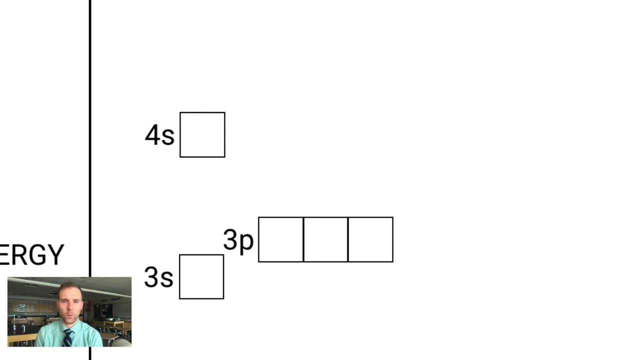 to start filling the fourth shell, the 4s subshell, than it is to finish filling the 3d subshell. let me say that differently: it's easier to start filling the fourth shell, even though we have more room to fill electrons in the third shell, and it's not until we've filled up the 4s subshell that we then go back. 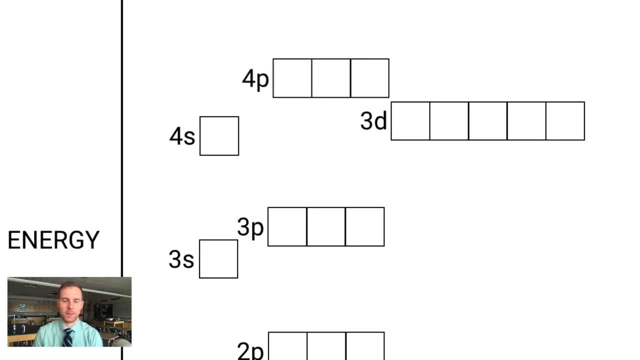 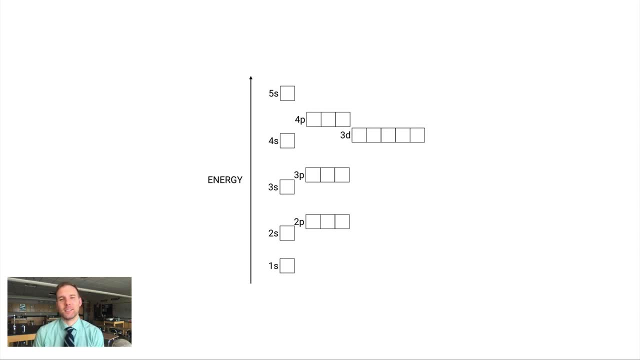 and kind of fill in the 3d subshell. once we get beyond that, we're now filling the 4p and then 5s, and this, this continues. so let's look at some examples, because i think that the best way to learn how this works is just to look at a bunch of examples. let's start with the most basic example. 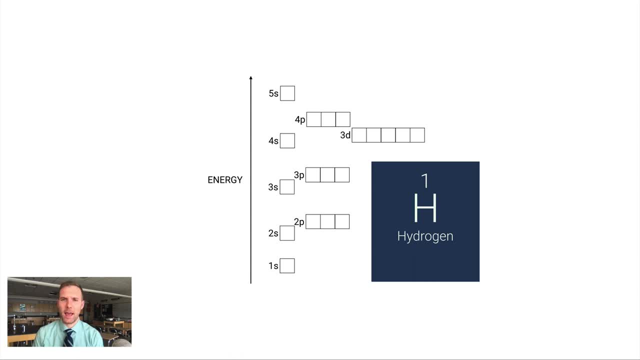 hydrogen. hydrogen only has one electron in it. if we're talking about an atom of hydrogen, so that one electron. i would fill in the 1s subshell. uh, i put it in as an arrow because electrons have a spin and so it's helpful to just see an arrow as opposed to a dot. uh, we'll talk. 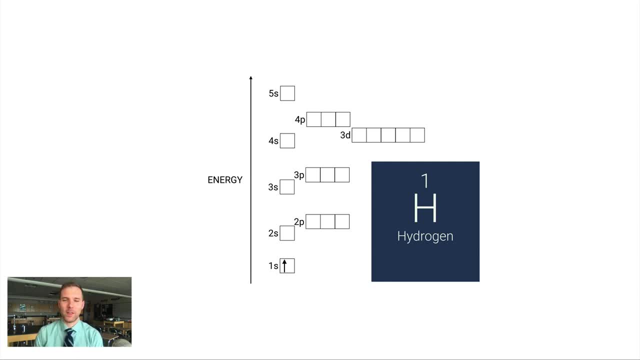 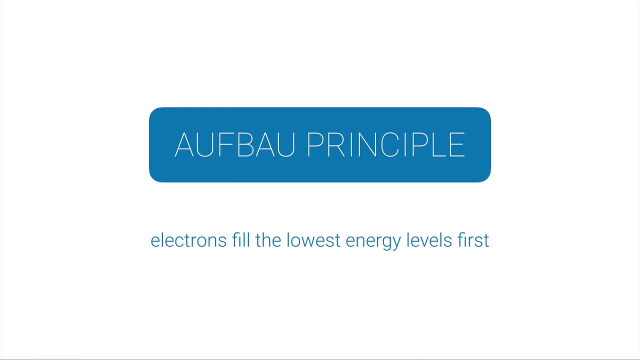 more about that in just a second. but i want to start with the 1s subshell, and that's because there's a principle or a rule we have to follow, and it's called the aufbau principle. aufbau is german for build up. and we're going to start with the 1s subshell, and that's because there's a 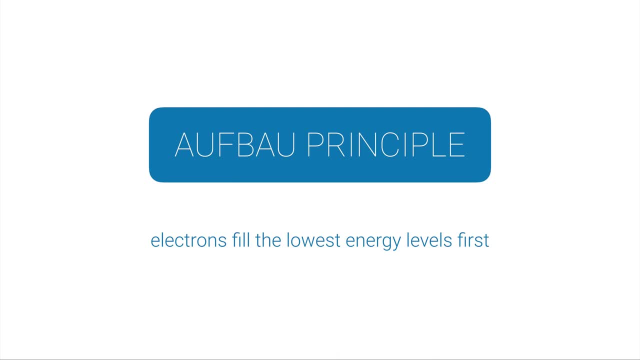 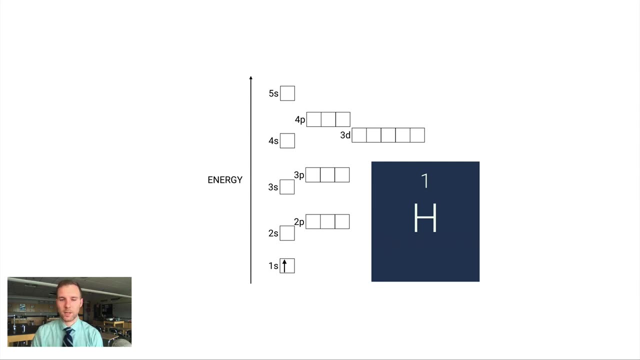 principle called the aufbau principle. and what the aufbau principle says is that electrons will fill the lowest energy levels first before they move on to higher energy levels. so that's why hydrogen would just have one electron in the lowest energy level, 1s in that orbital. now what's? 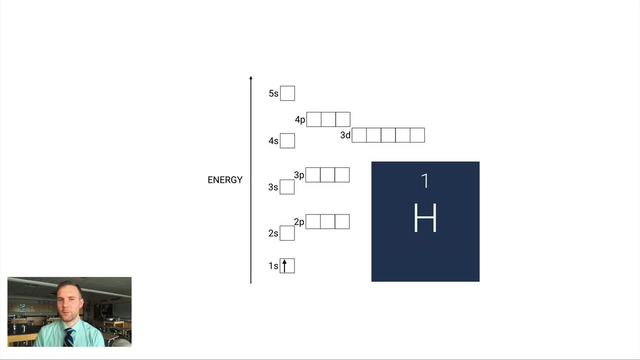 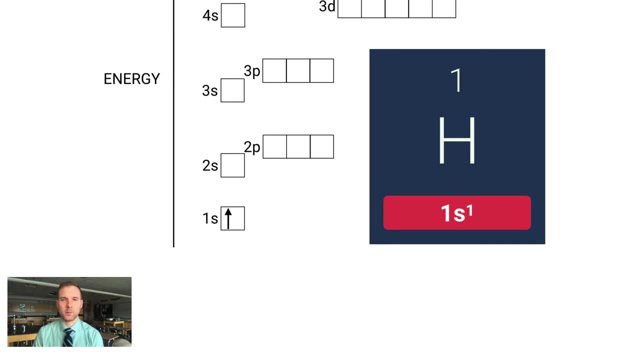 the electron configuration. well, there's a slightly different format. when we know this much information about the electron configuration, we'd write it as 1s, with a one subscript or one in the power. it almost looks like, and here's the breakdown for that: 1 is the shell, one through seven, s is the subshell of that shell. so 1s, the 1s subshell and then the. 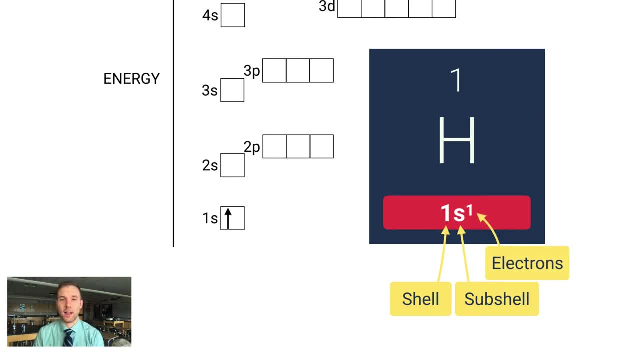 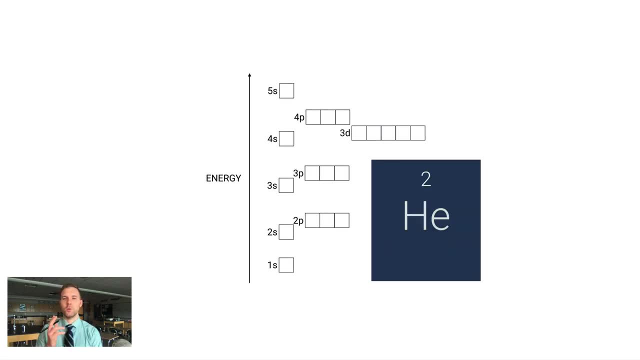 baby numbers as superscripts. those are the electrons. so 1s1 means that i have one electron in the 1s subshell. let's move on to helium. helium has two electrons, so i'm going to put one in 1s, just like i did for hydrogen. i have room for another in the 1s subshell, so the other electron. 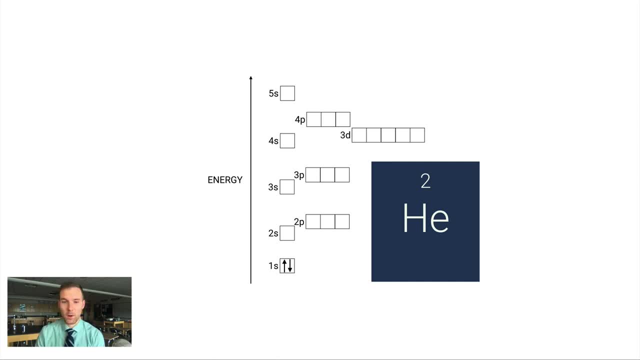 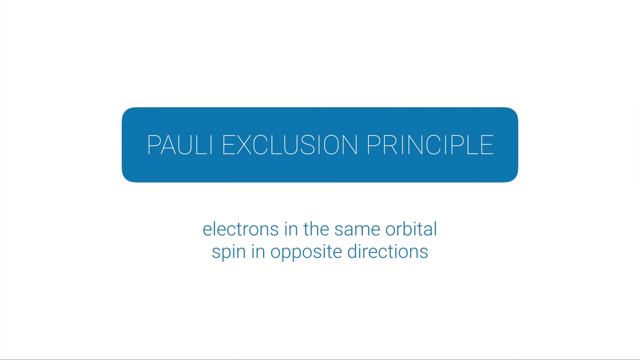 to make helium's two electrons is going to go also in that 1s subshell. now notice that arrow is pointing down and there's a reason for that. that's the, and the electron configuration would be 1s2. the reason for that arrow pointing down is the Pauli exclusion principle and this says that: 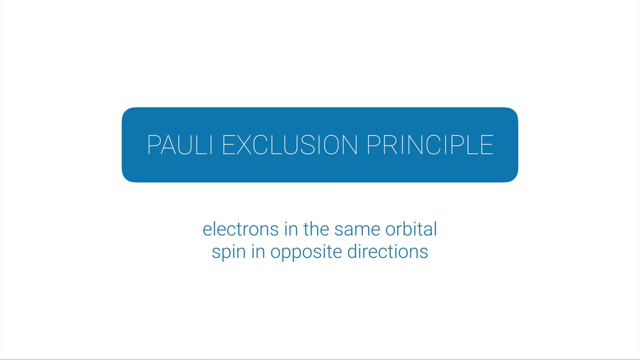 electrons in the same orbital will spin in opposite directions. keep in mind: these electrons are negative, and negatives don't want to be near each other if they don't have to. so spinning in opposite directions makes them a little bit more comfortable. let's move on to lithium. lithium has 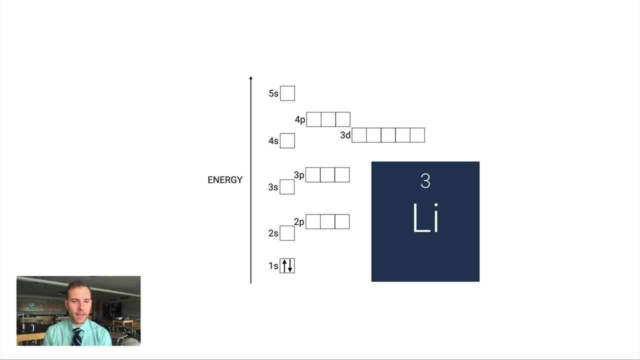 three electrons in it, one in the 1s, the other in the 1s. so now i've filled my 1s, i have to move on to the next highest energy level and that's 2s. so my configuration becomes 1s2- 2s1 if you look at. 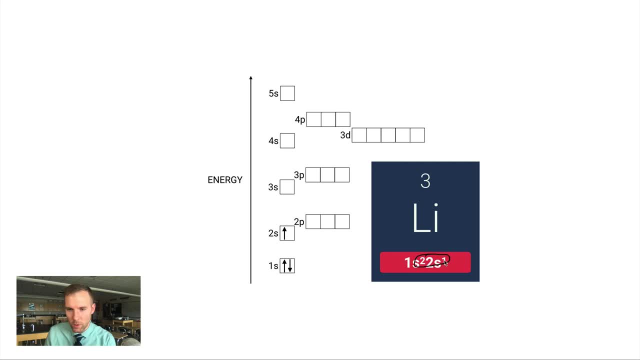 these baby numbers here, these superscript numbers two and one. that should always add up to three in this case, but really i mean generally it should always add up to the number of electrons that you intend on putting in the configuration. so that's a way to kind of check yourself. when you're done, let's move. 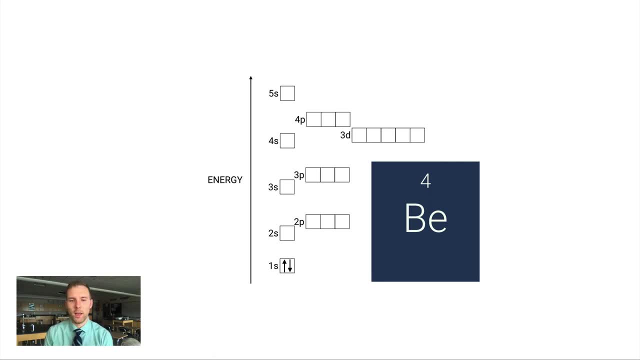 on to beryllium. beryllium has four electrons, two in the first shell, two in the second shell, and so this would just become 1s2- 2s2. starting to get the hang of this, let's keep going for another couple. 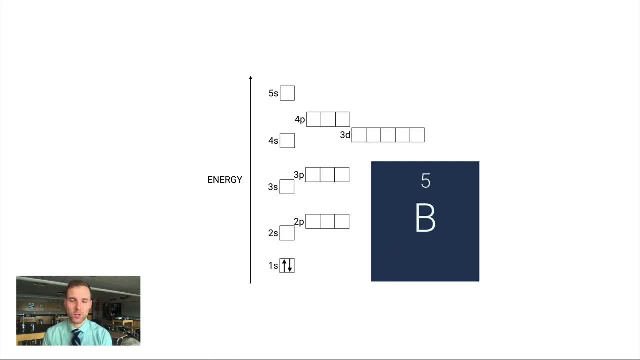 elements. boron has five, so two in the first shell, two in the 2s subshell and i'm not going to move on to 3s because the 3s subshells are going to be in the first shell and i'm not going to move on to. 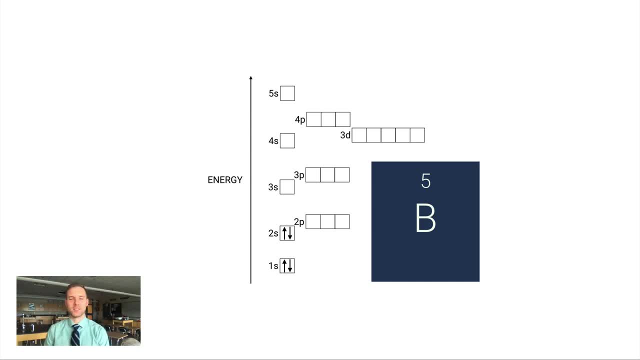 beryllium. beryllium is going to be in the second shell, so i'm going to move on to beryllium beryllium. so i'm going to start filling the 2p subshell, so this would become 1s2, 2s2, 2p1. okay, let's move on. 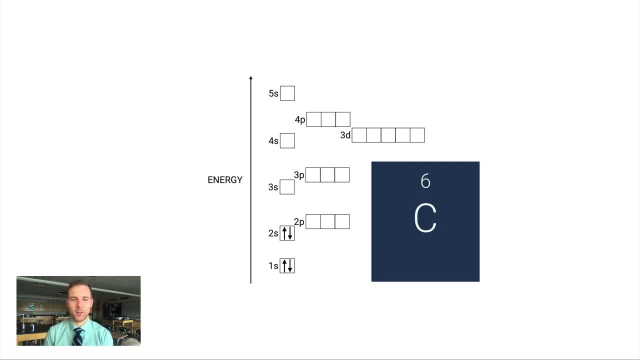 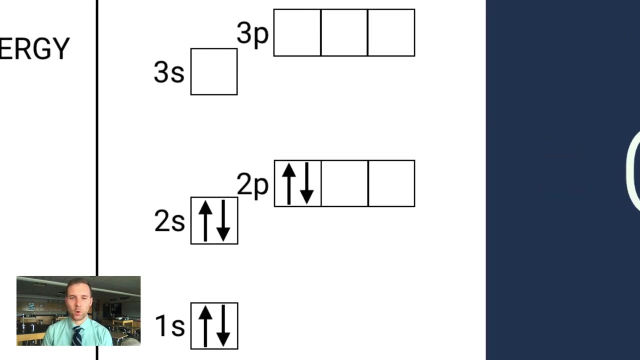 to carbon. carbon has six electrons, two in the first shell, two in the 2s subshell, and then you'd think that i just have two electrons here in the 2p subshell. and that's true. but the way that it's drawn out here, where both electrons are in the first orbital and the other two, 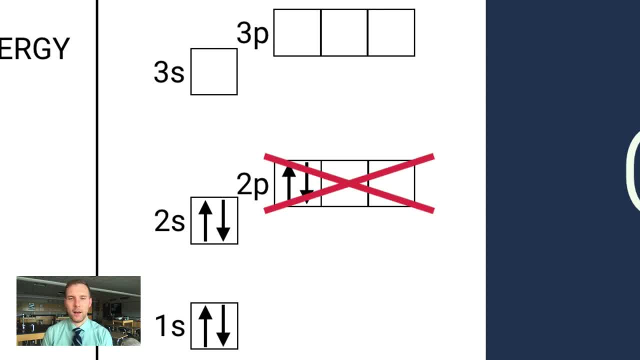 orbitals are blank. yeah, that's not going to happen. uh, imagine getting on a bus seeing that there's an open seat and there's a seat that has someone in it. you're going to go for the open seat before you're forced to buddy up with someone in a seat that's already occupied. this is called. 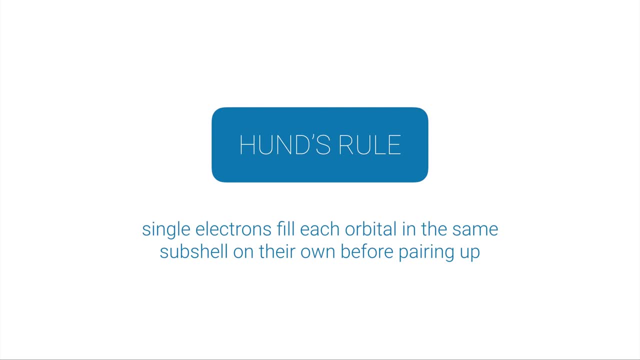 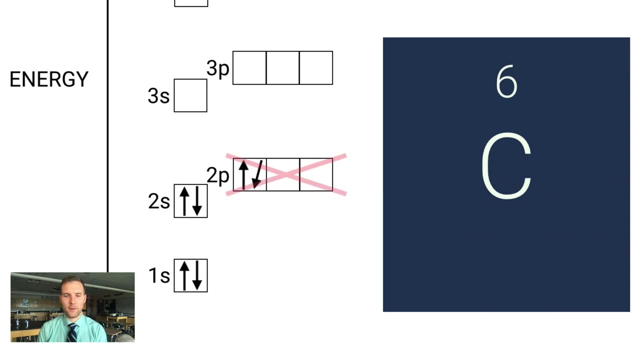 hun's rule. hun's rule essentially says that single electrons will fill each orbital in the same subshell on their own before pairing up, and so instead of having something like this, we'd have more something like that where we'd have, uh, still 1s2, 2s2, 2p2. but really we have to kind of know what's going on with these electrons here. 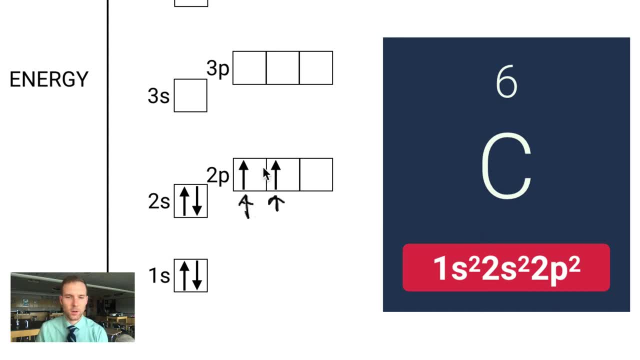 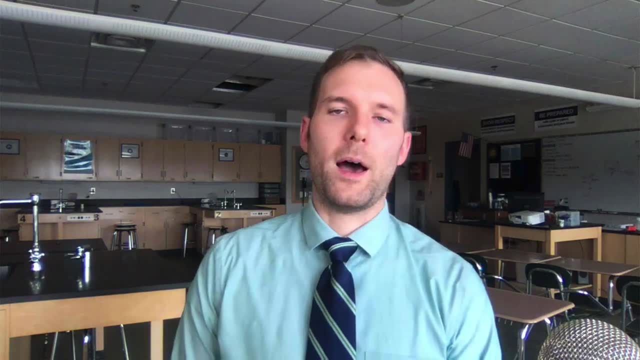 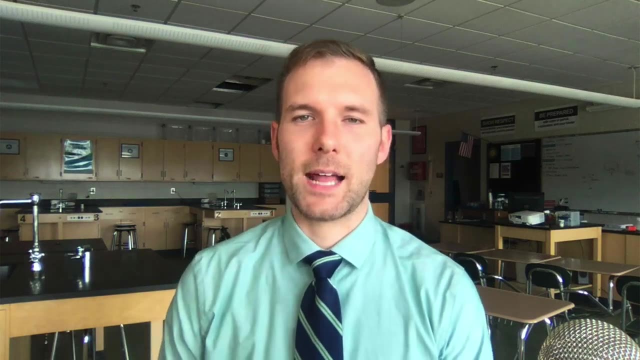 they're spinning in the same direction and they're not going to start to buddy up until they have to, okay, so let's uh, take a step back for a second. we've learned more about electron configuration, that we have a more specific, maybe advanced, way of saying exactly where the electrons are. 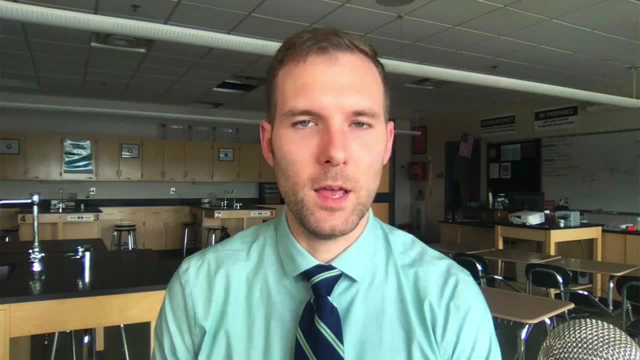 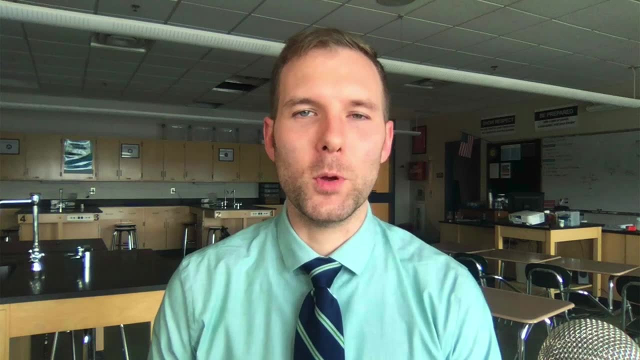 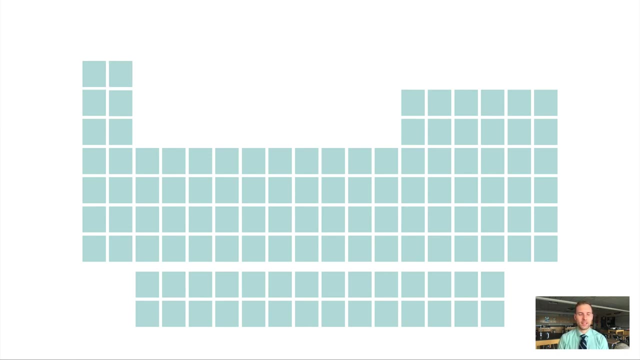 and sometimes this is the point where students kind of get pretty turned around and they start to think: how am i going to keep track of all of this? well, there's something that can help you immensely, and that's the periodic table. let me just slide helium over to right, next high, next to hydrogen, for a second, and then i want to kind of point out: 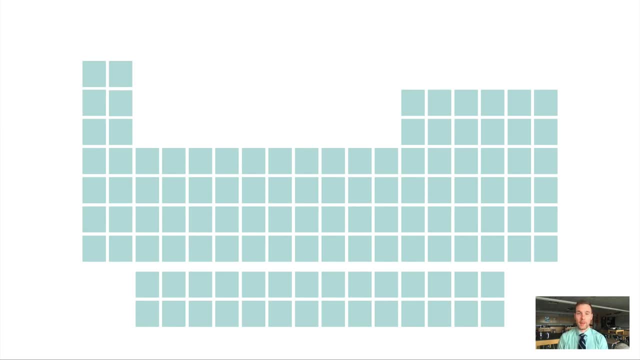 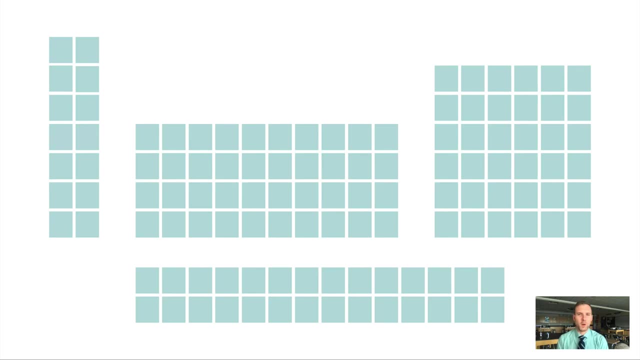 there's. there's kind of four areas of the periodic table that maybe you won't be able to unsee once you see it. let me kind of break out the periodic table a little bit. if you notice the first major flavor, psychosct phom Salt. 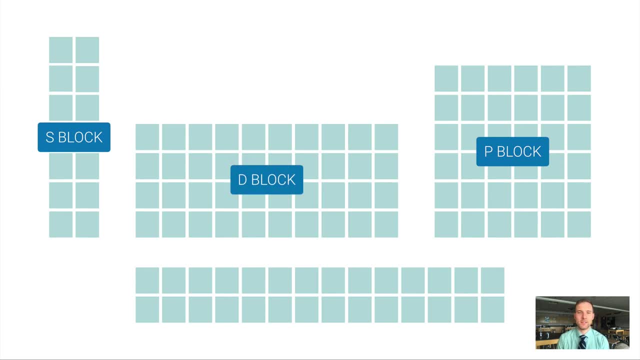 step three, equation phom Salt. In the center we've got 10 elements wide and that represents the D block or the D subshell, And then of course the bottom two rows there. that's the F block. If you count them up, there's 14 elements there. 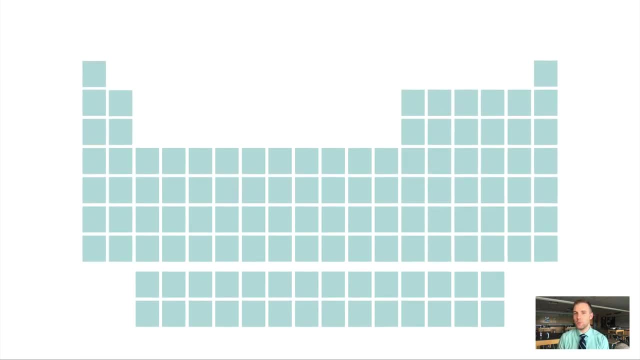 So I show you all of this to tell you that you can really use the periodic table to help you figure out what the electron configuration is for any element. Jump right into it. Let me show you hydrogen here. Hydrogens would be 1s1.. Heliums would be 1s2.. And then I'm going to just skip down to the next row here. Now I'm in the second shell of electrons. So lithium would have- this is just the end of its electron configuration: 2s1.. 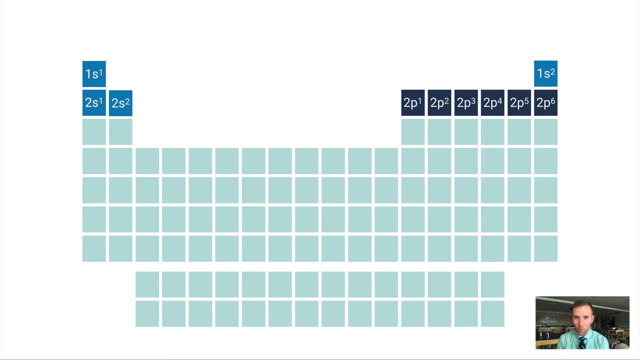 Beryllium 2s2.. Boron 2p1.. Carbon 2p2.. And I can keep going: p3, p4,, p5, p6.. Now my p subshell is filled. 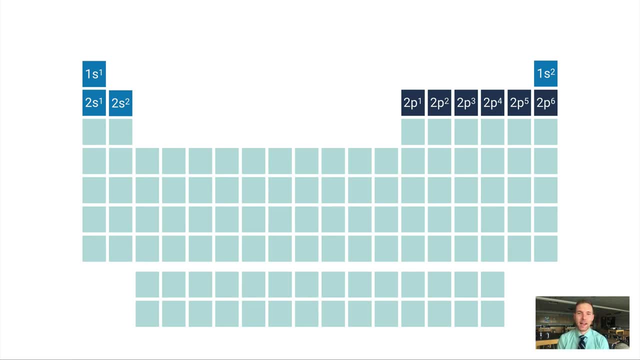 And what do you know? I'm also at the end of the periodic table. I now have to start over in the third row, just like I would move to the 3s subshell Now. there's nothing immediately next to 3s2.. 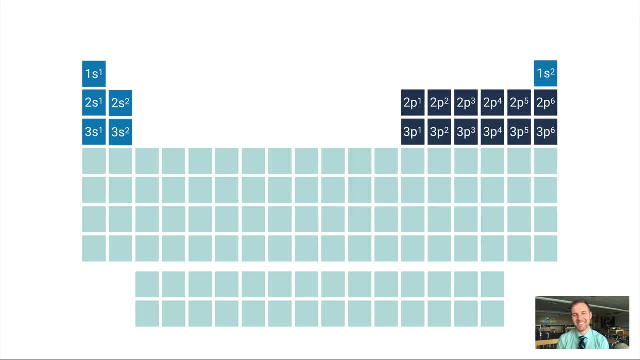 So I keep going over to 3p, 1 through 6. And then I'm in the 4s subshell. But now that that's filled I can then go back to the 3d subshell, And so that's where this 3,, this d block comes from. 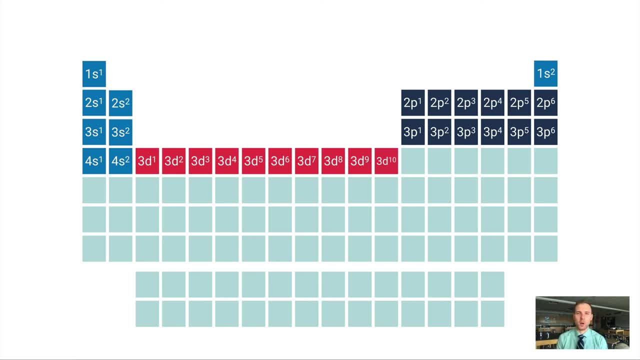 It doesn't match the row number, but you know that that's what we're doing with these orbitals. And then I can go back to the 3d subshell, And then I continue on with the 4p and so on. 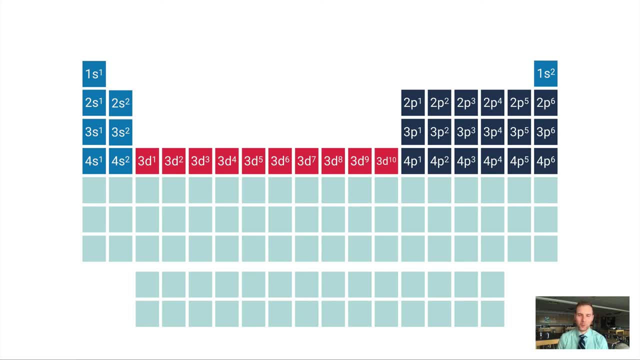 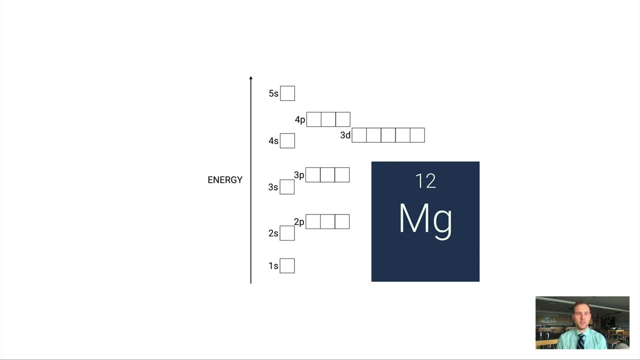 So the point here: the periodic table is incredibly helpful And the more you practice these electron configurations, I think, the more you'll realize that the periodic table is really truly a beautiful work of art and science come together. So I do want to show you some of these electron configurations can get pretty long. 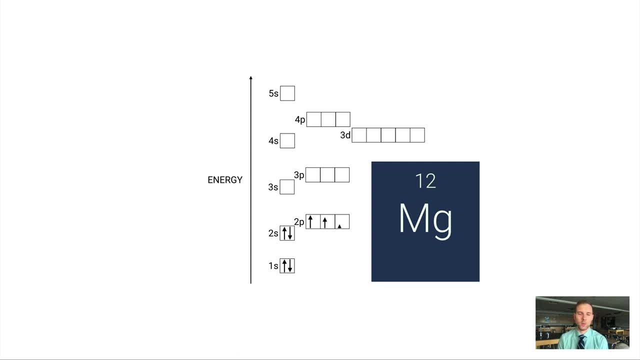 So let's look at magnesiums: 12 electrons mean: 2 in the first shell, 8 in the second shell, That's 2 in 2s and 6 in 2p, And then 2 in the third shell. 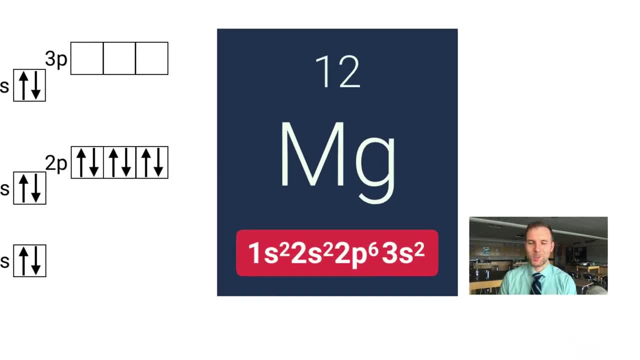 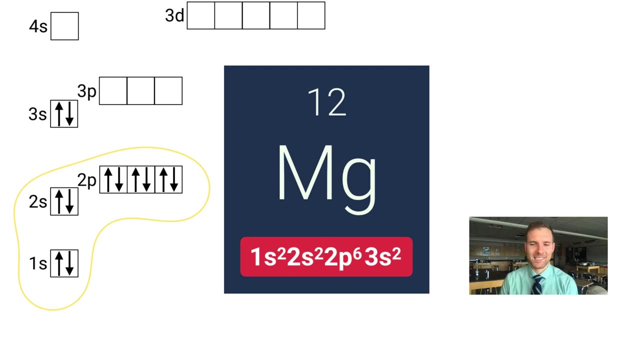 So the electron configuration is 1s2, 2s2, 2p6, 3s2.. That's a lot to say and it's a lot to write. So there's a trick I want to show you. If I just look at this piece here: 1s2, 2s2, 2p6.. 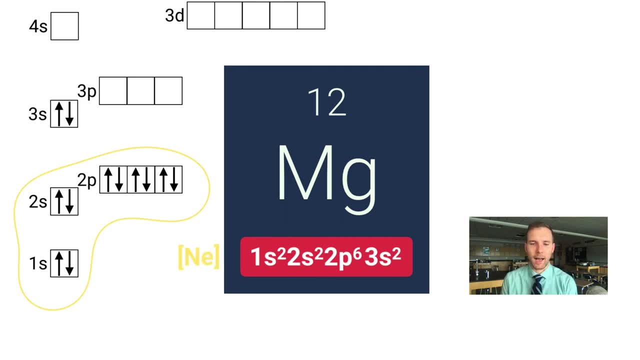 That is the electron configuration for neon, Neon being the most recent, The most recent noble gas that we would have gone through. It's at the end of that periodic table, all the way to the right. And think of this: like I have neon and then I just have two more electrons. 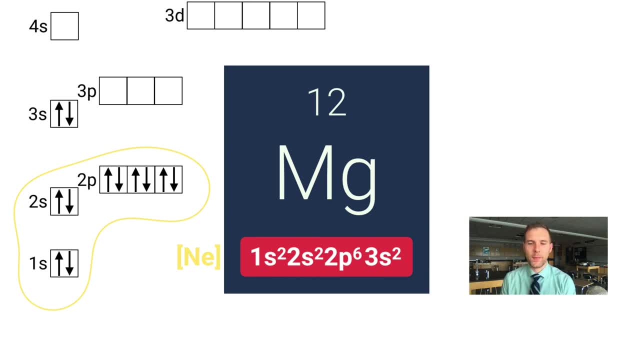 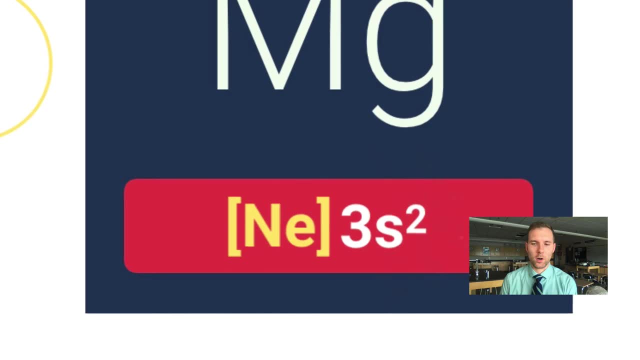 one in the 3s and the other in the 3s. If I can think of this this way, then what I can do- and I'm allowed to do this- is replace the neon configuration part of this with just neon's element symbol. 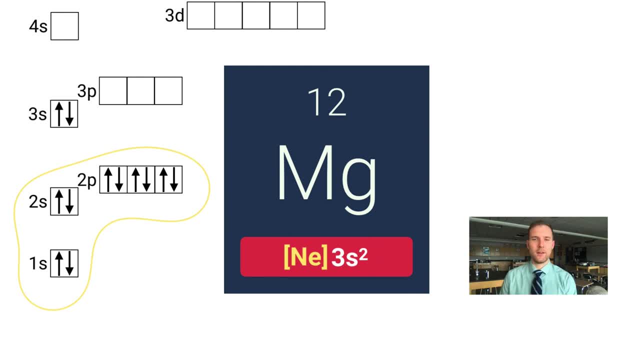 in square brackets like this. So this is a time saver. You go to Google and type in magnesium electrons Electron configuration. It's going to show you this instead of the full 1s2,, 2s2,, 2p6, 3s2.. 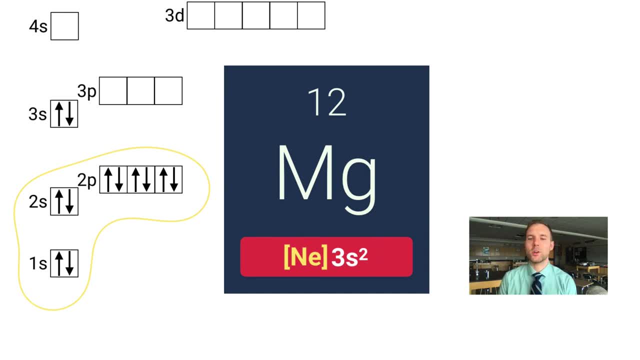 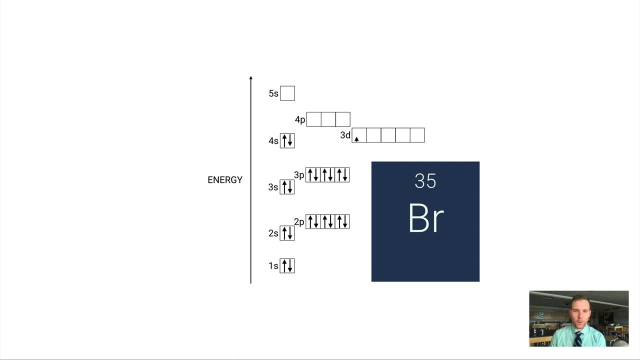 It's just going to show you neon 3s2.. Let me show you another example. Let's do bromine: 35 electrons Oof. Well, for that I'm just going to fill in all my electrons as it would normally fill in. 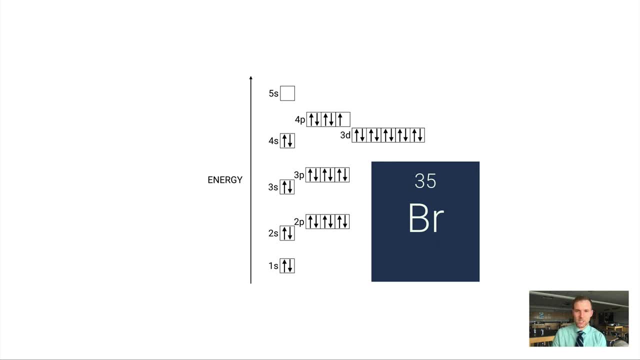 I've got all the way up to 4p5.. Well, this piece here from 1s2, 2s2, 2p6, 3s2, 3p6.. That would be argon. So this here is argon. 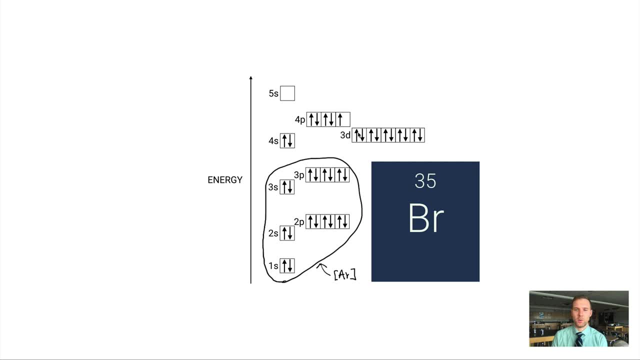 And then I just pick up from where I left off: Argon 4s2,, 3d10,, 4p5, just like this here. So this is called the noble gas shorthand trick or noble gas configuration. This is something that you want to use really when you get beyond. 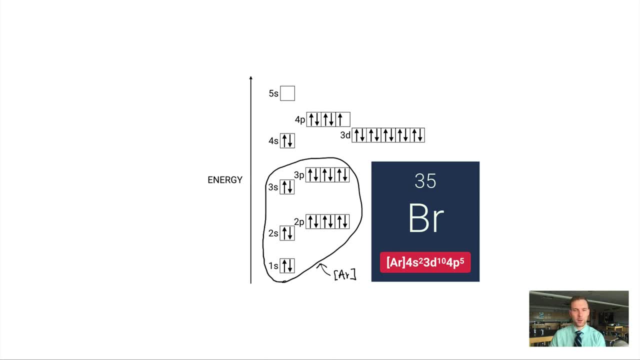 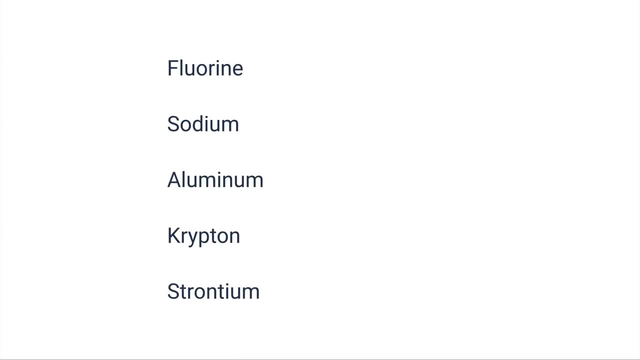 probably when you get beyond neon. to be honest, You probably wouldn't want to use it when you get beyond helium, because that's just 1s. So let's put this all to the test. Here are five atoms. I want you to just write the electron configuration down on a scrap piece of paper. 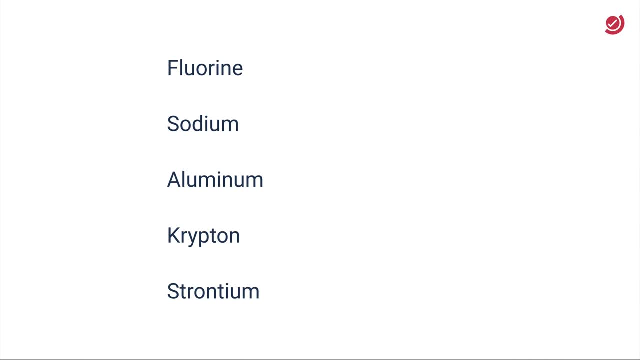 And I'll show you the answers once this little timer icon in the top right corner goes out. Okay so, fluorine 1s2, 2s2, 2p5.. Notice, I can kind of check this by just looking. 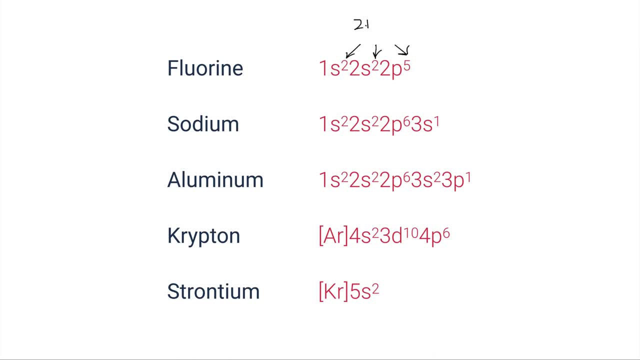 All right, 2 plus 2 plus 5, 5 equals 9.. And that's how many electrons? And that's how many electrons are in a fluorine atom. When you finish writing electron configurations, I'd always recommend you check these to make sure they match how many electrons you want to put in. 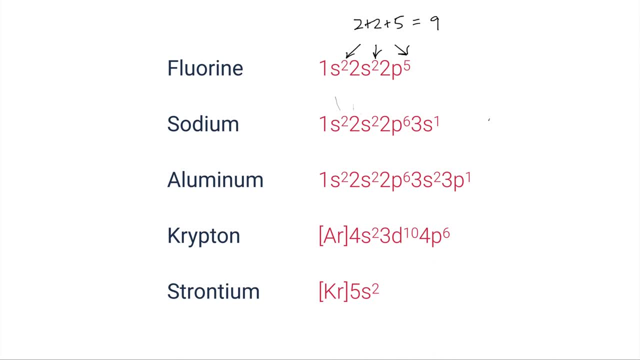 Sodium would be 1s2, 2s2, 2p6, 3s1.. That should be a total of 11 electrons. This right here is shorthand for electron Aluminum: 13 electrons: 1s2, 2s2, 2p6, 3s2, 3p1.